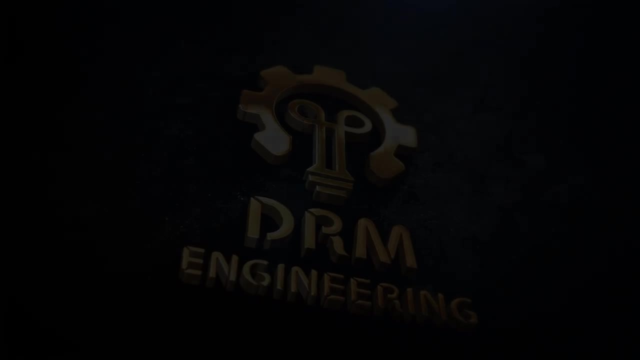 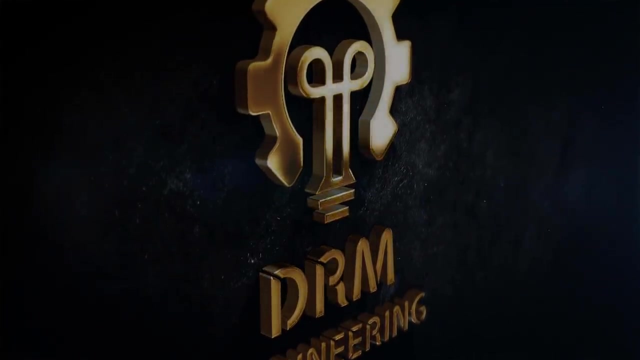 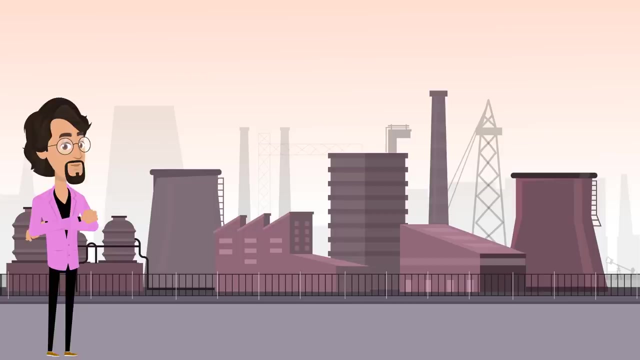 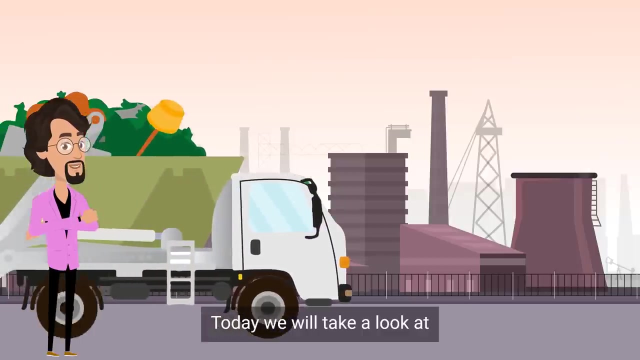 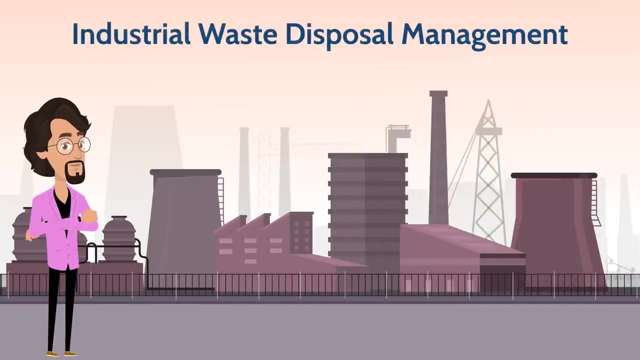 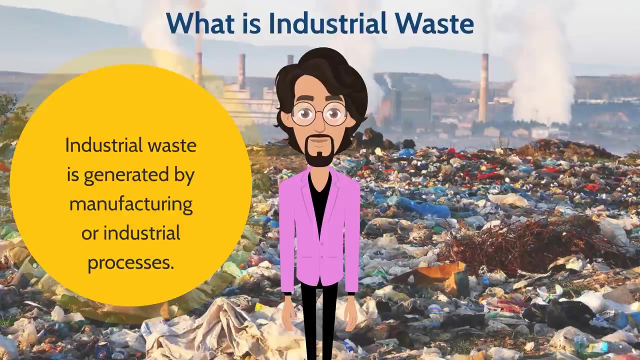 Hi everybody. I welcome you all to today's video. Today we will take a look at Industrial Waste Disposal Management. Come, let's get into the video. Industrial waste is the waste generated by manufacturing or industrial processes. The types of industrial waste generated include cafeteria garbage, dirt and gravel masonry. 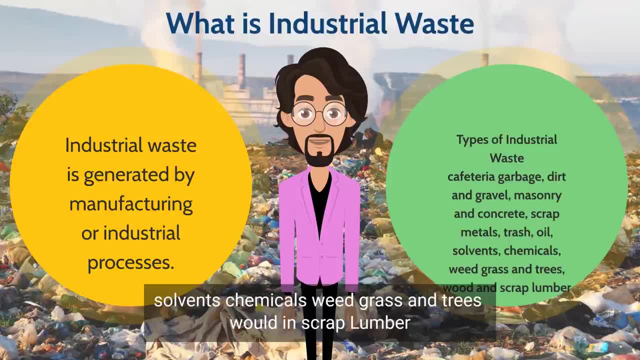 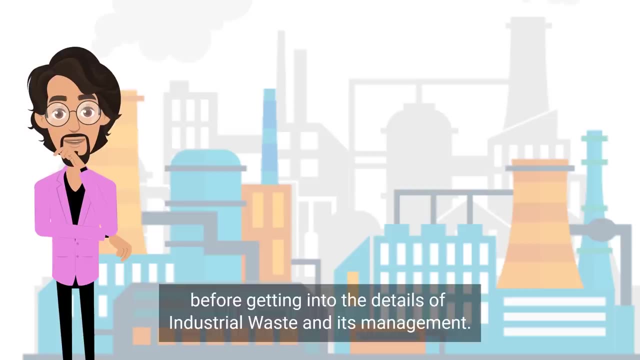 and concrete scrap metals, trash oil, solvents, chemicals, wheatgrass and trees, wood and scrap lumber and similar wastes. The disposal of industrial waste in the right manner is a vital process. Before getting into the details of industrial waste and its management, we need to know three key words. 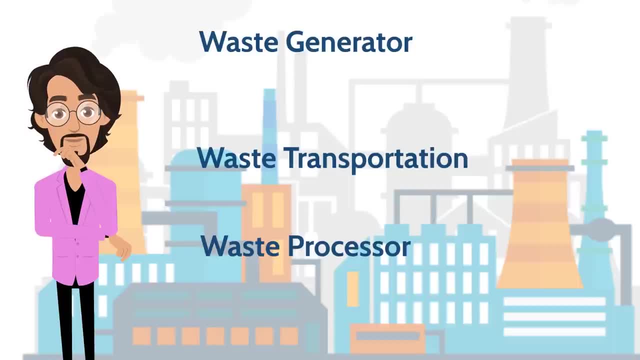 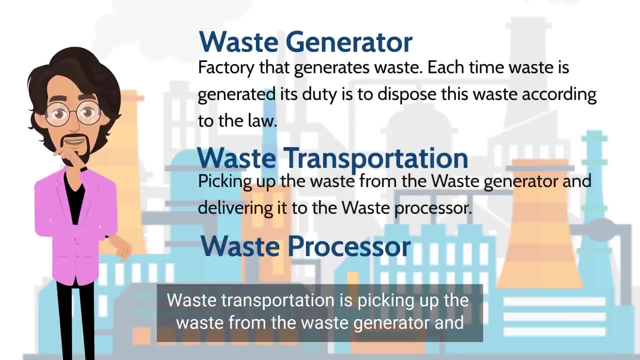 Waste generator, waste transportation and waste processor. Any factory or industry that generates waste is a waste generator. Waste transportation is picking up the waste from the waste generator and delivering it to the waste processor- A factory that treats, disposes or recycles waste. 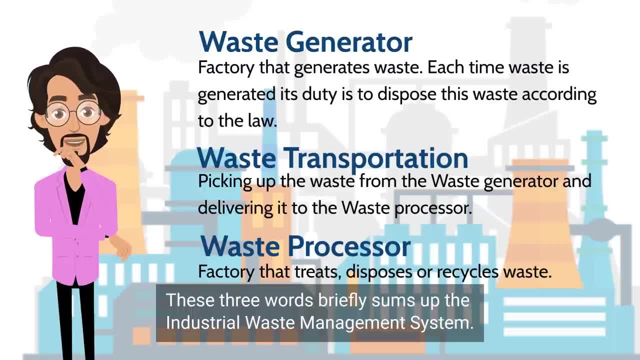 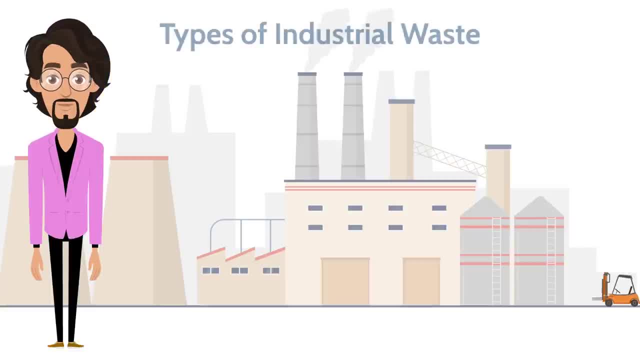 These three words briefly sums up the industrial waste management system. Now let us see these in detail. Now we will take a look at the different types of industrial waste. Industrial wastes are of four types: Liquid waste, solid waste, chemical waste and hazardous waste. 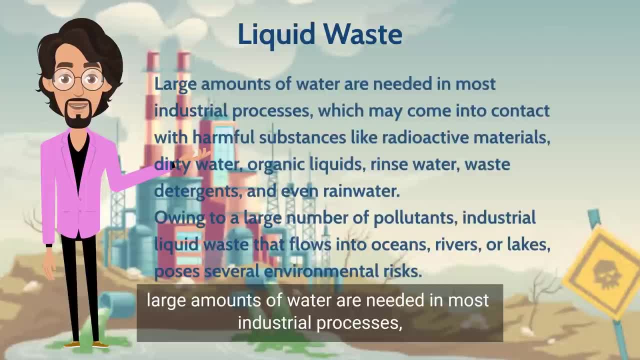 Liquid waste is produced industrially. Large amounts of water are needed in most industrial processes, Which may come into contact with harmful substances like radioactive materials, dirty water, organic liquids, rinse water, waste detergents and even rainwater, Owing to a large number of pollutants. industrial liquid waste that flows into oceans, rivers. 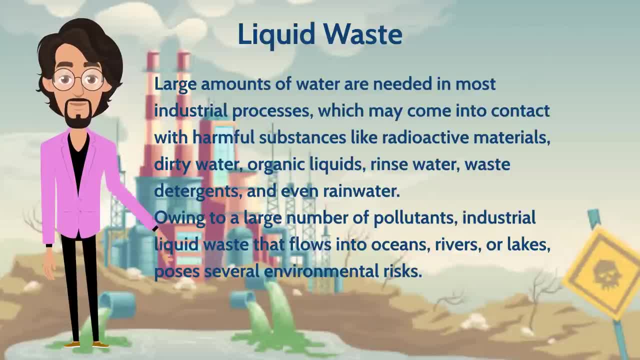 or lakes poses several environmental risks. Businesses and factories are required to install wastewater treatment facilities To stop the polluted water from flowing into large bodies of water, since if it flows in untreated, it could harm the surrounding environment and, in severe cases, even the 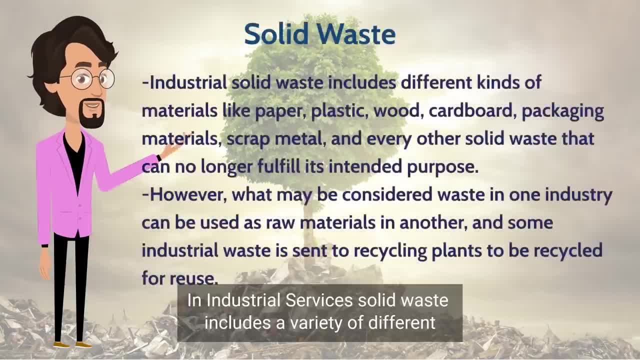 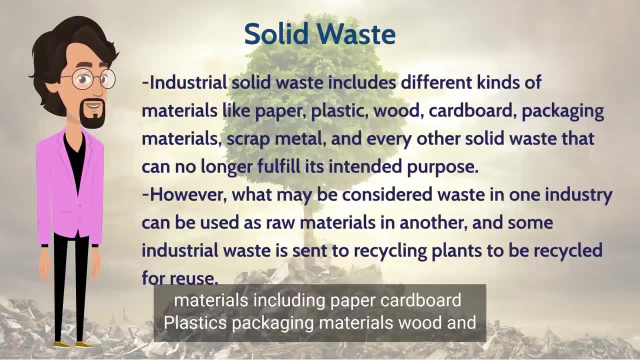 surrounding population. In industrial services, solid waste includes a variety of different materials, including paper, cardboard, plastics, packaging materials, wood and scrap metal. Some of these materials can be reused and recycled by a recycling center. A recycling center can process the majority of industrial solid waste, effectively reducing 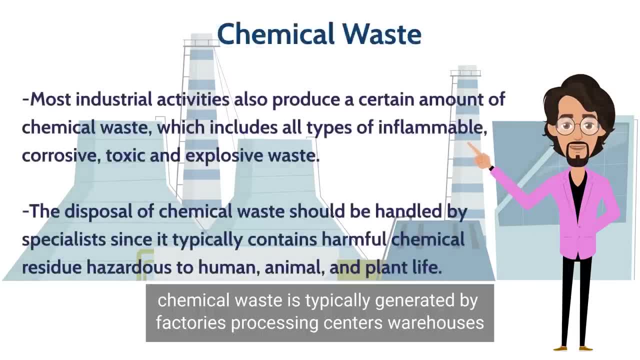 your waste disposal costs. Chemical waste is typically generated by factories, processing centers, warehouses and plants. This waste may include harmful or dangerous chemicals and chemical residue in waste disposal. Chemical waste must be segregated on site And waste disposal may need to be handled by a specialist to ensure compliance with. 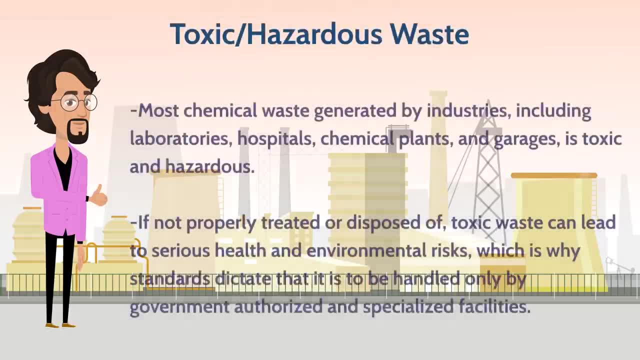 health, safety and legal requirements. Toxic and hazardous waste is comprised of materials that can cause pollution. pollution and pollution problems cause serious health and safety problems if waste disposal is not handled correctly. this type of waste typically includes dangerous byproducts, materials generated by: 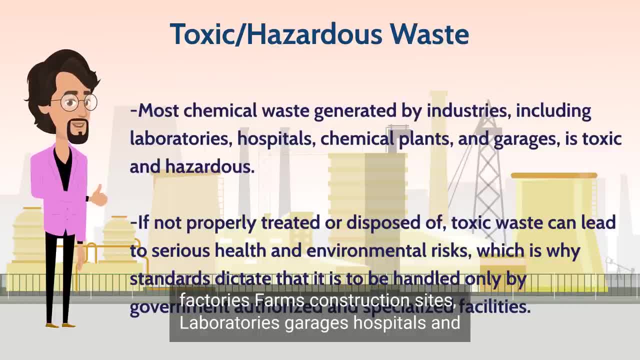 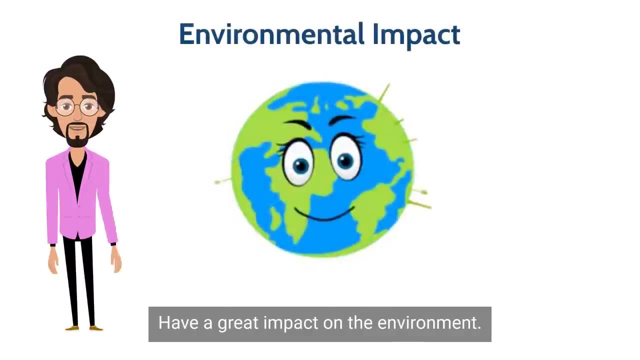 factories, farms, construction sites, laboratories, garages, hospitals and certain production and manufacturing plants. this waste disposal is only legal at special designated facilities around the country. these industrial wastes have a great impact on the environment. factories and power plants are typically located near bodies of water due to the need for large 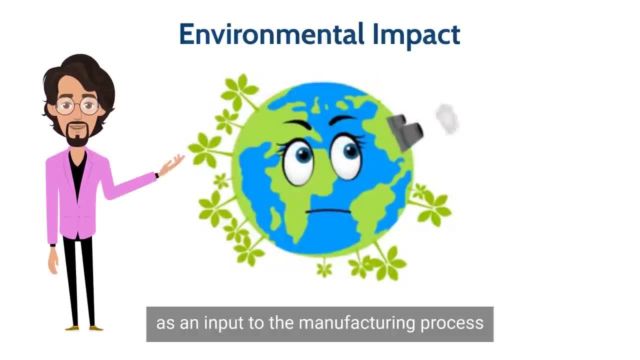 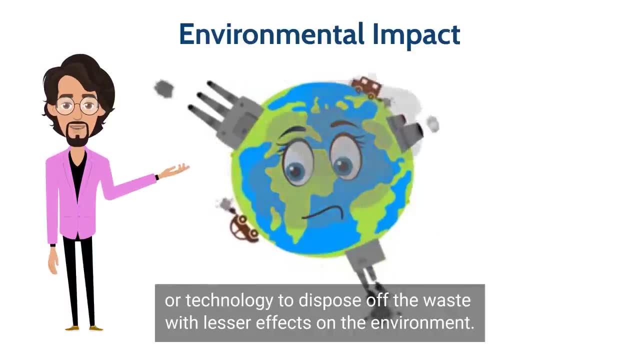 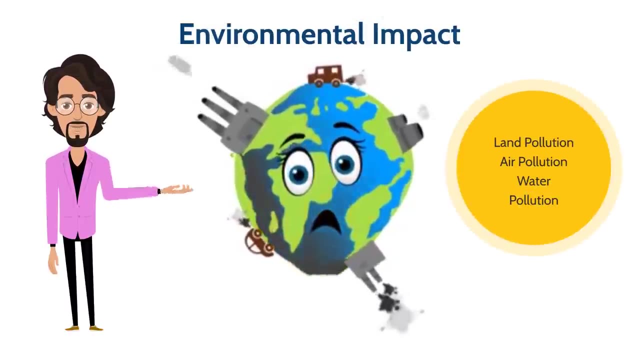 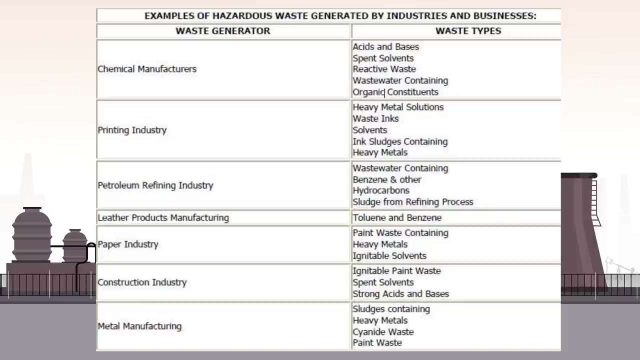 amounts of water as an input to the manufacturing process. many areas that are becoming industrialized do not yet have the resources or technology to dispose off the waste. with lesser effects on the environment. they cause land, air and water pollution. they can be disposed of at the cost of a large amount of waste. 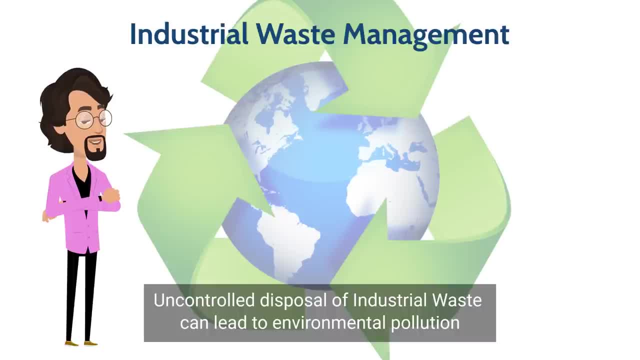 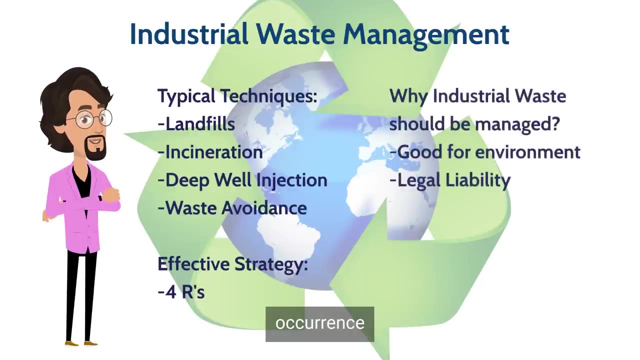 uncontrolled disposal of industrial waste can lead to environmental pollutions and irreparable damages. the soil, water and air near industrial waste dump sites are regarded to be very harmful to animals and humans. as such, disposing of industrial waste the right way will prevent against such occurrence. manufacturers are governed by policies that require them to dispose of. 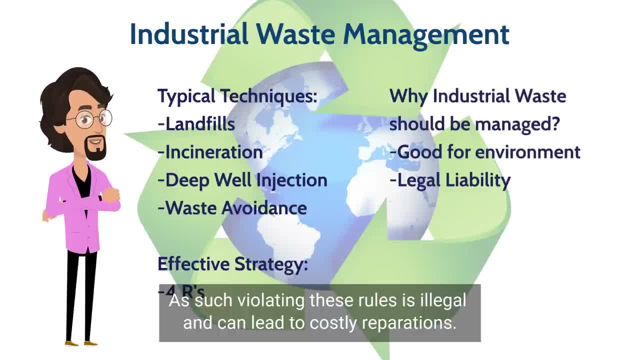 industrial waste the right way. as such, violating these rules is illegal and could lead to costly reparations. managing industrial waste is one of the ways to protect our environment from harmful pollutants. as such, manufacturers and companies should be held responsible for the waste they generate. the industrial waste management system works like this: 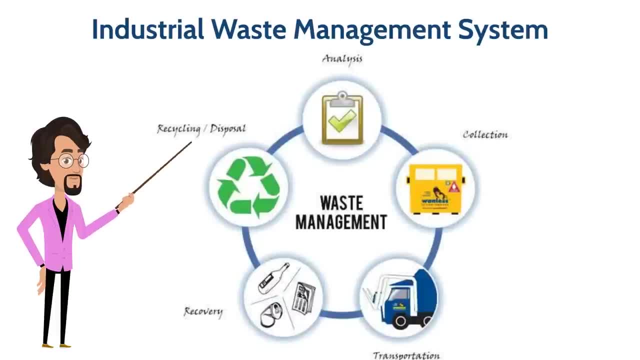 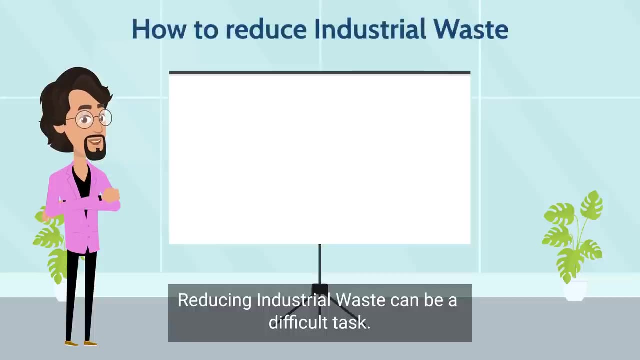 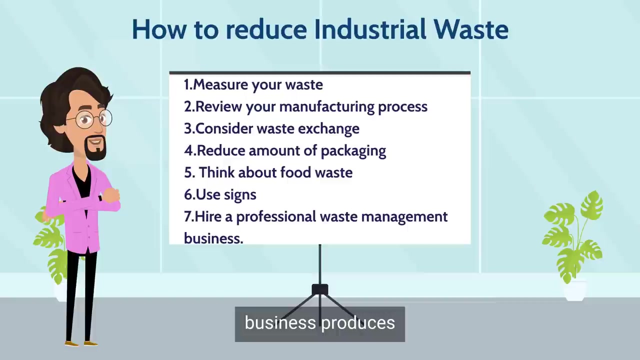 first the waste is analyzed and segregated. then the waste is collected from the factory, the suisth process. the waste is then transported to the waste processor. these wastes are then recycled or disposed accordingly. reducing industrial waste can be a difficult task. there are many reasons why you should both reduce. 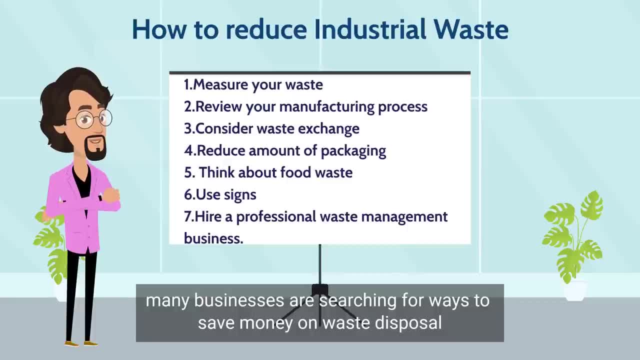 the amount of waste your business produces. firstly, there is the financial cost. many businesses are searching for ways to save money on waste disposal. disposing of waste can get very expensive. You should reduce the amount of waste your business produces. And the amount of waste that your business sends to landfill is the environmental cost. 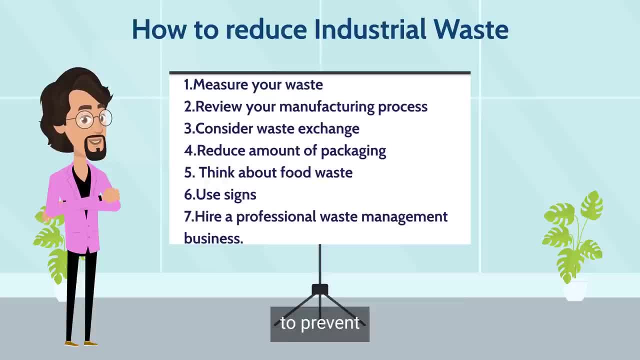 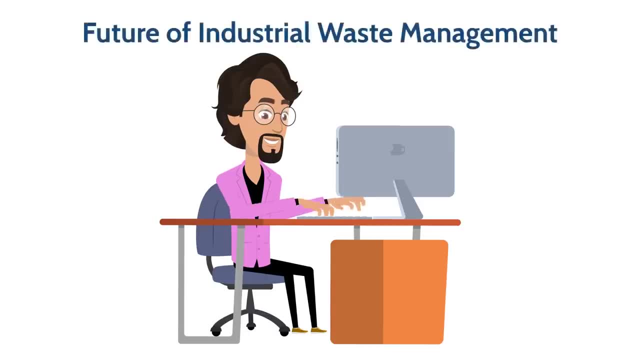 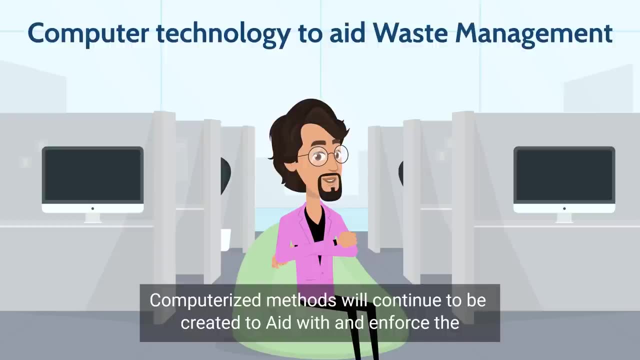 Our environment is precious and it is important that we do everything possible to prevent or minimize any harmful effects that our activities may have on the environment. Computerized methods will continue to be created to aid with and enforce the division of waste from recycled materials. This includes using robots at recycling facilities to sort the waste- GPS-operated compactors. 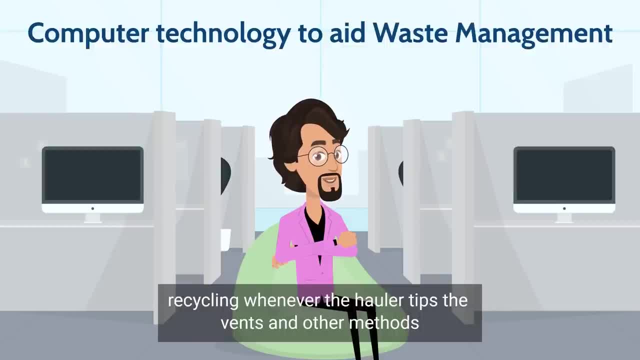 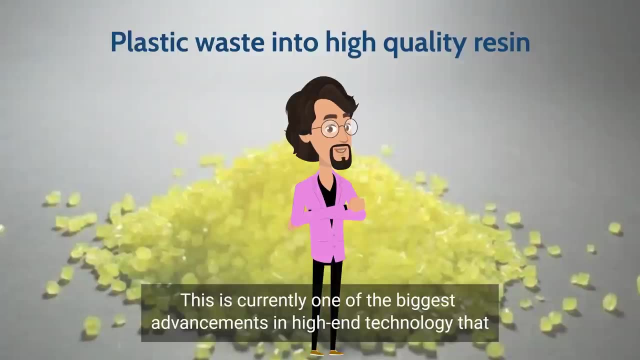 chipped recycle bins that record which households are recycling whenever the hauler tips the bins, and other methods. Researchers will develop new technologies to locate unconventional recyclables, such as wasted food, on-site. This is currently one of the biggest advancements in high-end technology that is happening in. 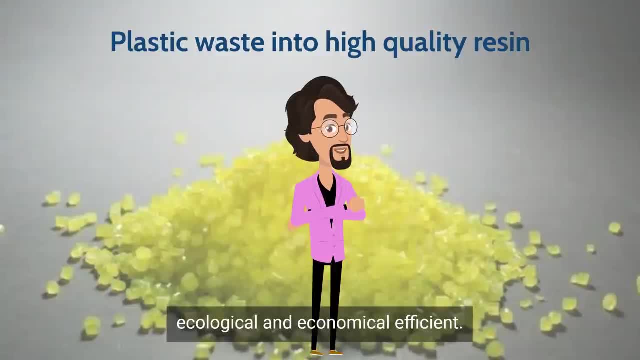 the management of solid waste, Ecologicalscom, Ecological and economical. efficient plastic waste is turned into high-quality resin. The process emits less greenhouse gas than is emitted when making prime resin. Though currently ahead of the game, this is one area that the industry will need to continue.